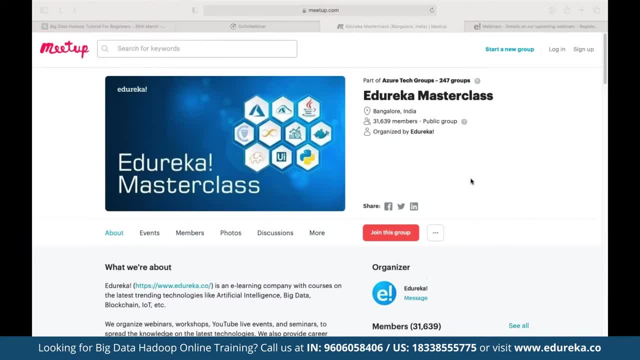 masterclasses, we conduct multiple webinars and live events on different topics, including blockchain, IoT, artificial intelligence, machine learning, big data and multiple front end and back end development technologies. And the best part about these seminars are they are absolutely free of cost, So there are no hidden charges involved here. So, as 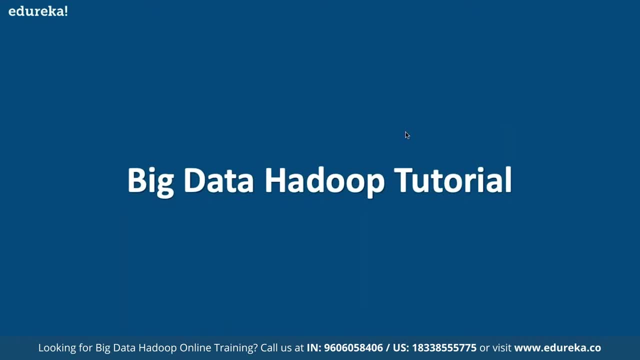 a part of our discussion here today. we are: we have gathered for our discussion on top of big data tutorials. So we have- we are going to discuss on the components of big data, what exactly it is, and then we are going to talk about what exactly is big data, big data, 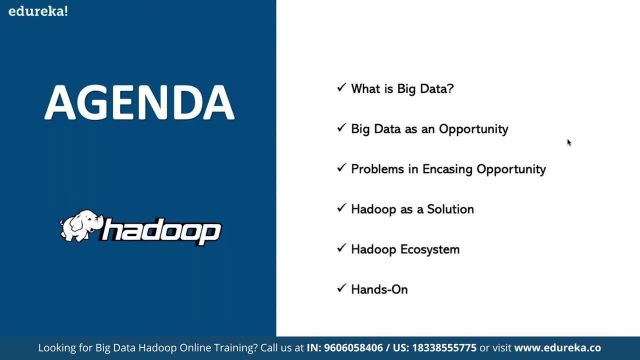 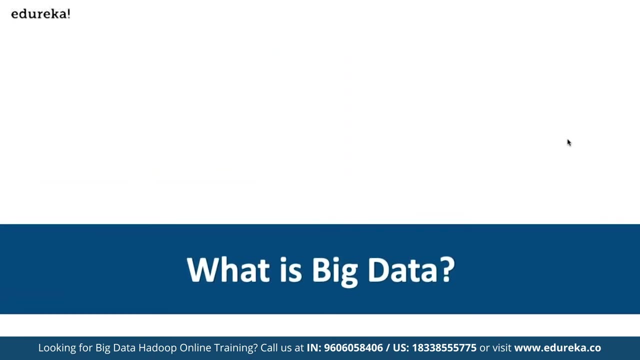 as an opportunity, and then the problems and encasing opportunity here: Hadoop as a solution and Hadoop ecosystem itself, And then we are going to talk about the hands on, if possible. So, basically, what does that be big data is so big data is what big data in simple layman terms, it's required for. 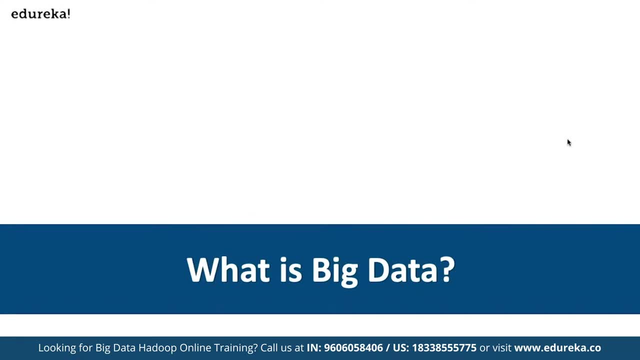 processing large amount of data. Now for a project to be classified as big data, we need that project. How, having more than 1000 GB in size, then only it is going to be considered as a big data project, right? So any, any data size having less than 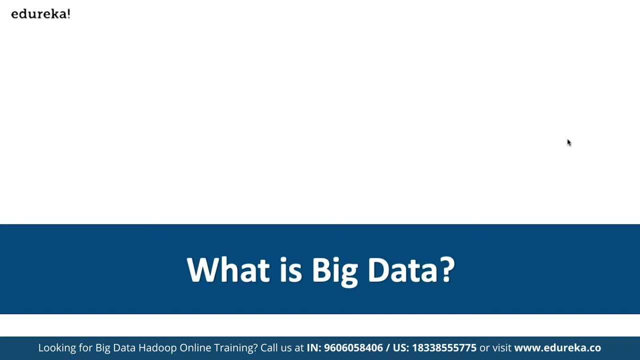 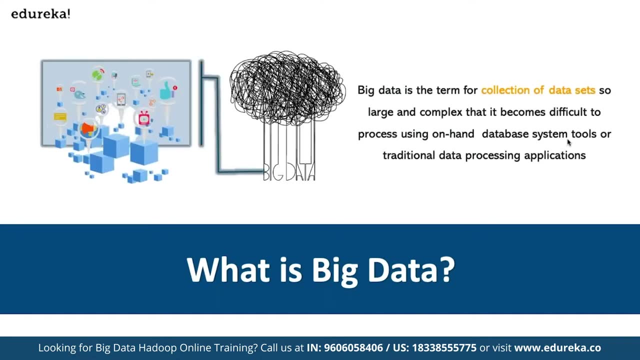 1000 GB is not going to be considered as a part of big data project. And big data is what? in simple layman terms, it's a process of reducing the time required for processing large amount of data set, For example, let's say, for processing. we need, let's say before. 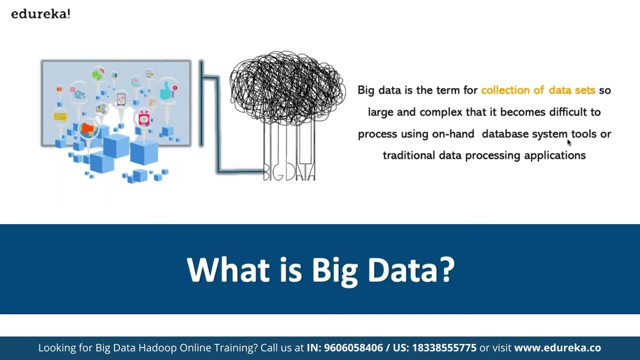 processing, let's say, 100 GB of data, we need 10 days. So instead of doing that, we can reduce the time here to do a few hours to a few minutes as well, by using the concepts and the tools available under big data components. So that is actually what it is. So, basically, 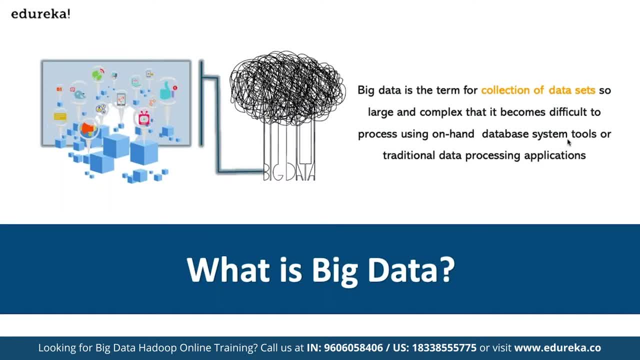 if you remember the last time we had used floppy disk, right. so again, early, we used to have floppy disk or a CD to store data, right? So let's say they were sufficient to handle the data, amount of data at that point of time. But again now data is currently. 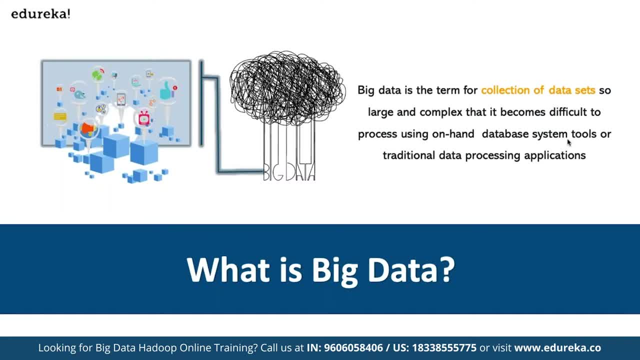 growing at an exponential rate, right, And that's why people are storing data in relational database systems as well. But again, with the increase in the amount of data set, the need for having a better insight of data is also going to be increased. That means now, 80% of data is currently generated. 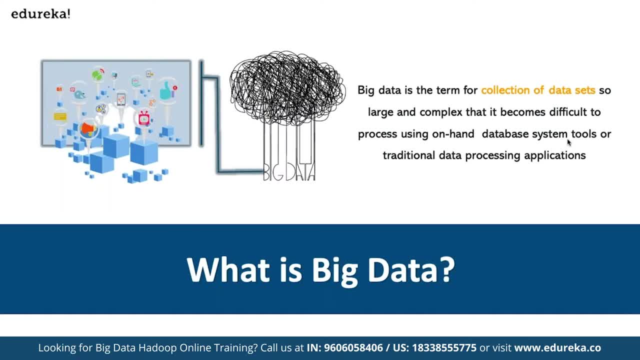 in terms of the unstructured data formats. That means when we say unstructured data, we mean audio clips, video files, images, and these are considered as unstructured objects, And 80% of data right now is all unstructured, thanks to all the social media platforms that. 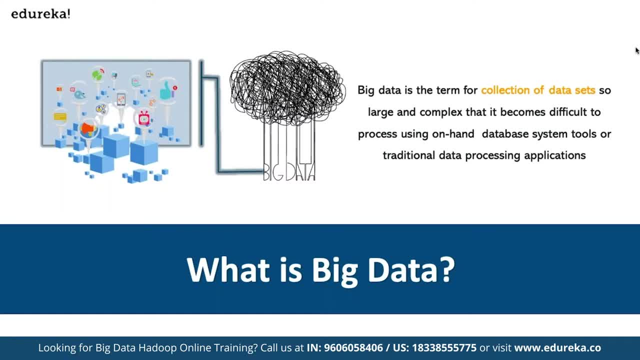 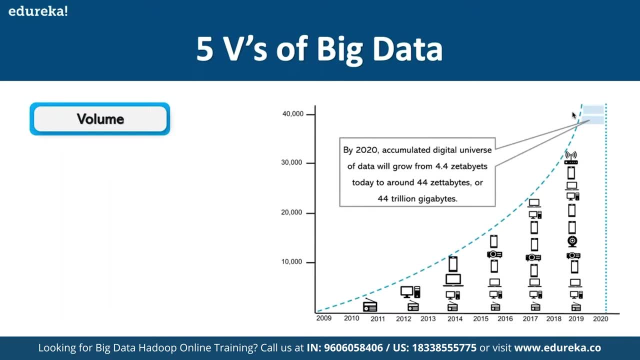 we have, And that is what Big Data helps us in analyzing these kind of unstructured data set. So there are five V's of Big Data. We have volume. So by 2020, accumulated digital universe of data will grow from 4.4 zettabytes to create around 44 zettabytes or even 44 trillion gigabytes. 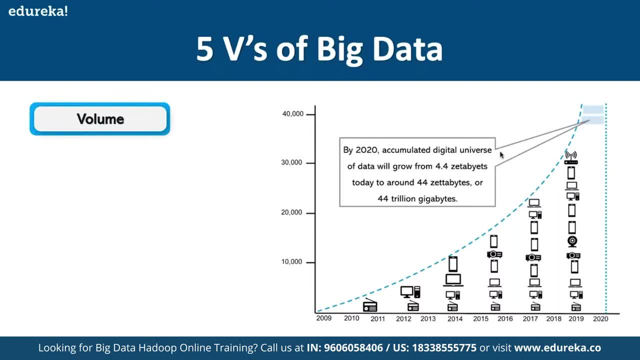 as we can see here, And by next four years it is going to be increased to 100 zettabytes on a per month basis. So, and that has been an exponential growth In terms of amount of data being generated on a per month basis, all thanks to 4G revolution. 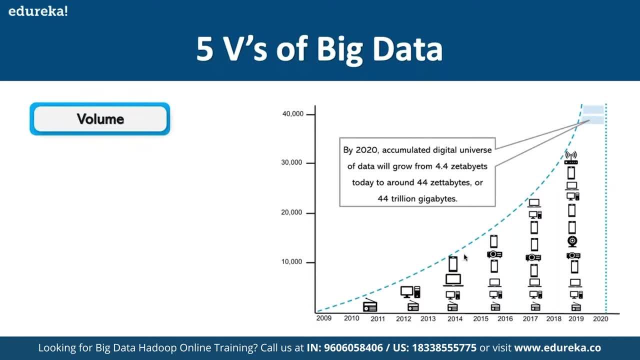 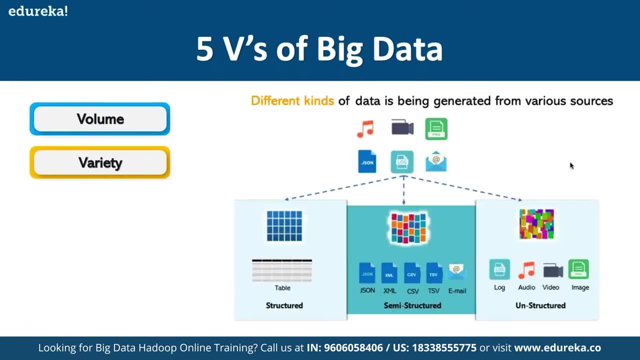 which happened back in 2016.. And because, from that point onwards, the data has increased multiples. right, Then we have variety. So in terms of variety, we have to. So basically, here we focus the data in terms of different coming in different formats. 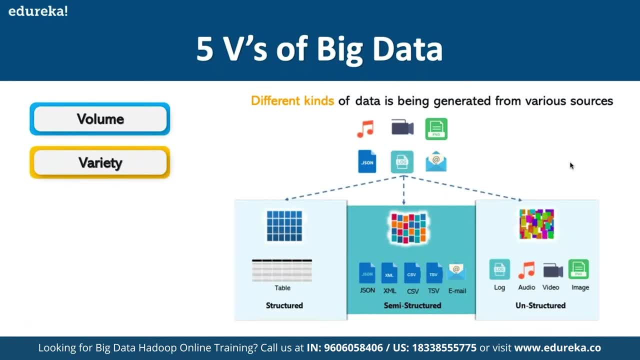 So variety means what the data is in different formats. We have the structure database, We have the semi structure, We have unstructured data set as well, Correct. So basically, in terms of all structured, we know we mean our DBL or we need DBMS databases. 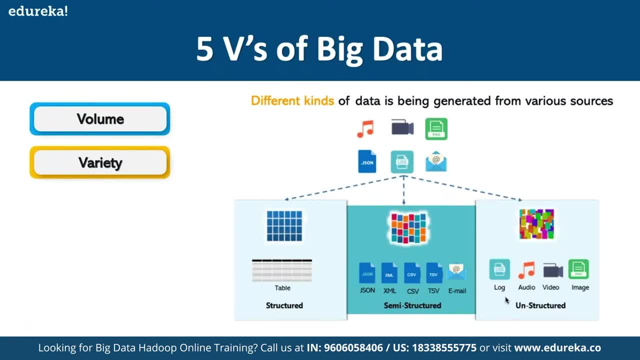 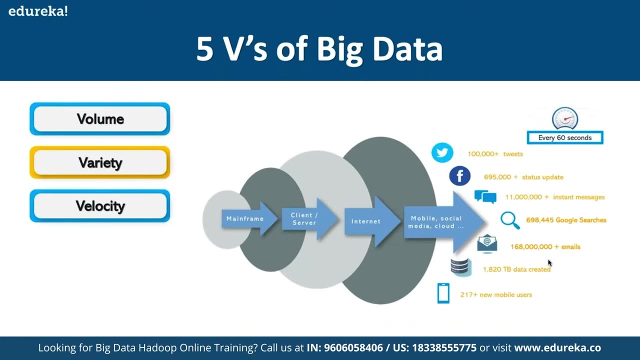 We have semi-structural and we have emails, CSV files, We have a JSON, scripts, XML files, and then we have unstructured, which is basically all the multimedia elements, And then we have velocity. So velocity, that means the rate at which data is currently being generated. 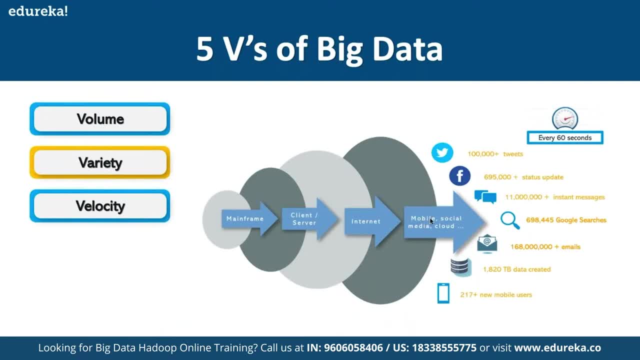 So we know that in terms of mainframe clients. So as far as the data on the upfront server, Internet, mobile, social media platforms- again they all are generating humongous amount of data on a per second basis. They all are generating humongous amount of data on a per second basis. 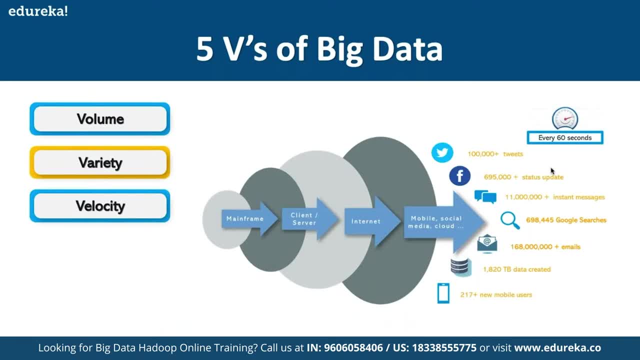 And that's why, again in terms of these sales, I'd be here in them. So the instant messages: we have to make sure that we do have the system to handle this much of data, and that too, which is being generated at an exponential rate. 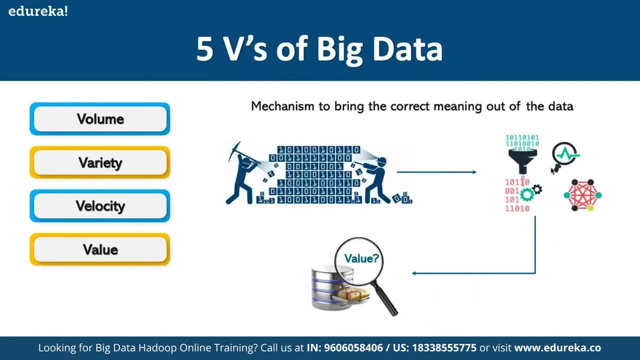 And that is what again is handled by beta documentation. Data is just data component itself and here we have value. so basically, when we are doing something, we have to first of all, before we start doing something, we have to evaluate: is that worthwhile? that means 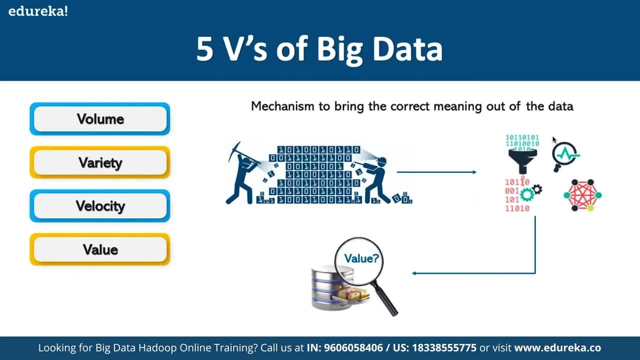 if we are going to invest time in doing that activity, is it going to be worth it, right? so, if that so, that is why we have to also evaluate the value. that means what is the value of data that we are going to value of information that we are going to get from this data set? if the, if the? 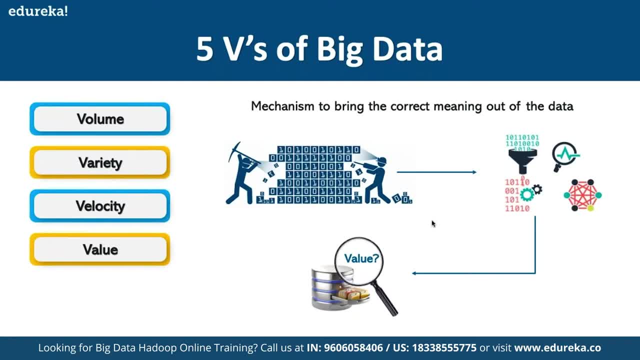 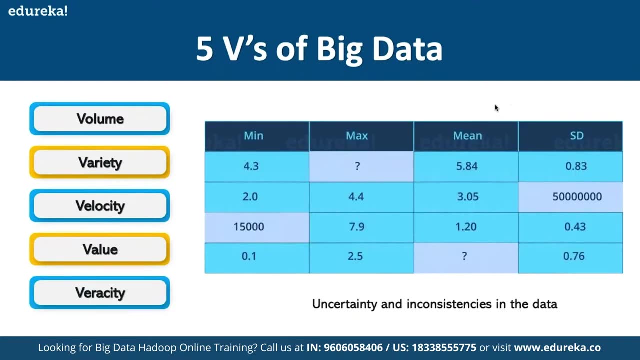 value is not going to be higher than the time and resource invested in solving, in mining the data, and that then then there is no use of big data there, right? so value has to be there, else it is not going to be feasible for us to mine the data right. so now we have big data as an opportunity. 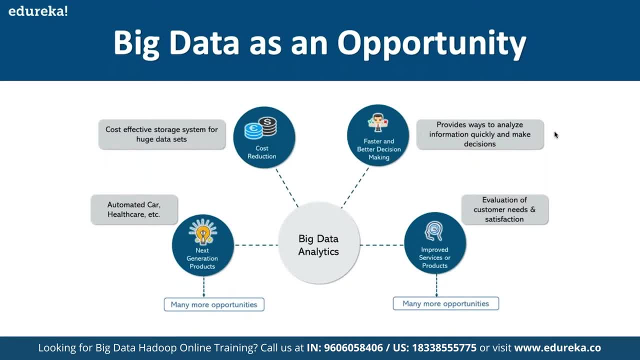 so big data, again analytics is cost effective because, again it's so. it allows us to store, it allows us to show humongous amount of data set right. it has multiple opportunities in terms of the next generation of products because, again here, for creating something for the r? d part, we have to make use of multiple data. select we. 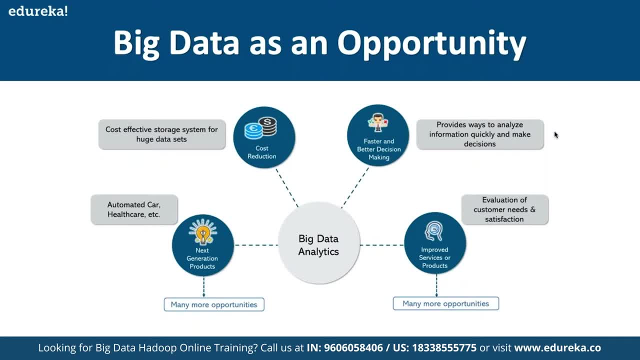 have to take care of the data being generated in automated in automotive industry, in healthcare, where we have humongous amount of data already already just being there, and then we have to make sure that we have the data set right so that we have the data set right, so that we have the data. 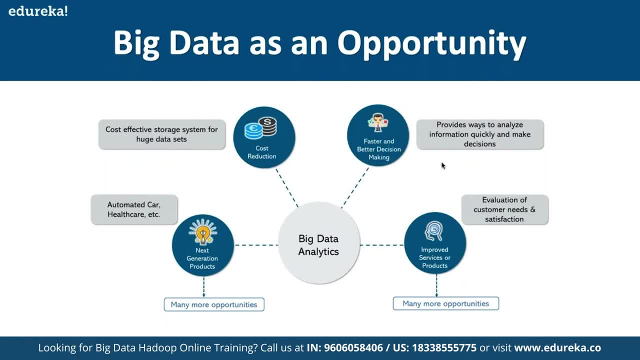 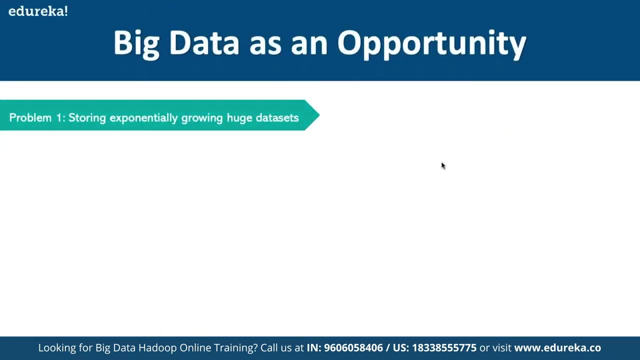 sure we are able to provide ways to analyze information quickly and make decisions. we should be able to improve services and products as a part of evaluation of customer needs. and now the problems with encasing opportunity. here is so. the first problem is we have a huge problem in storing exponentially growing, huge data set. so data generated in past two years. 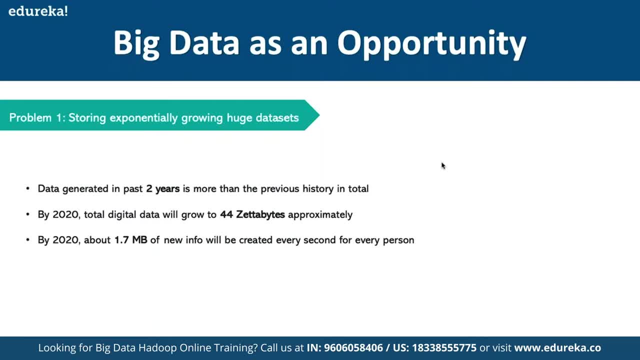 is more than the previous history in total. that's something to say, and again, but again by again, by the next year itself. so again it says 20, 20, but again by next two years it is going to grow more, somewhere around 80 zettabytes approximately, this might be. 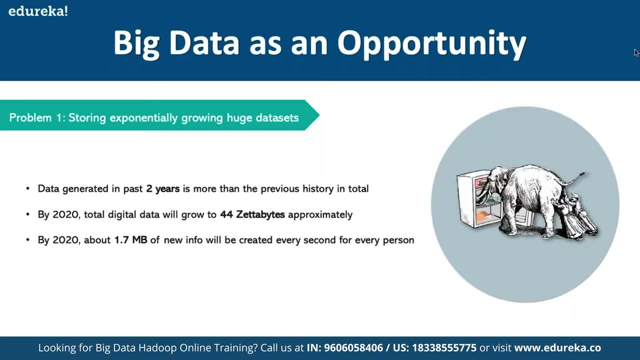 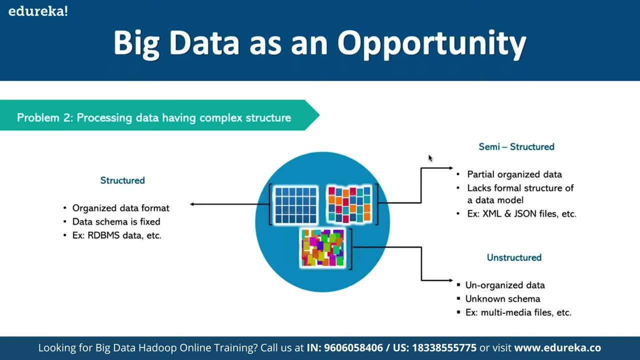 within next two years and that's why it has to be generated. and the second problem statement we have: it is going to be structured, for example. here we have to have a structured, organized format. that means data needs to be again different formatio in terms of rdb's data sets. here 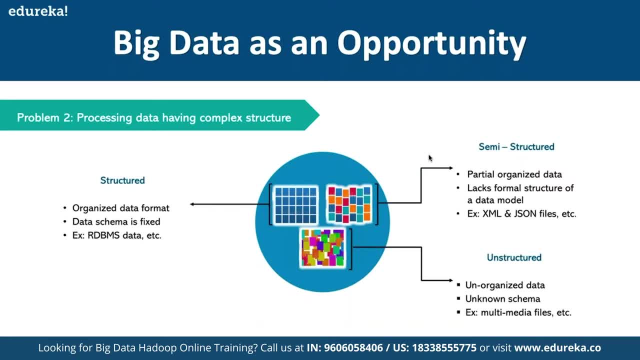 we're having a fixed schema, whereas, in terms of the seven, structured have partially organized data which lacks formal structure, and then, in terms of unstructure, we have all the multimedia files here. so now we need to have different ways of analyzing and handling different files, and that is what we have to make. that is what we have to focus on by using big data. 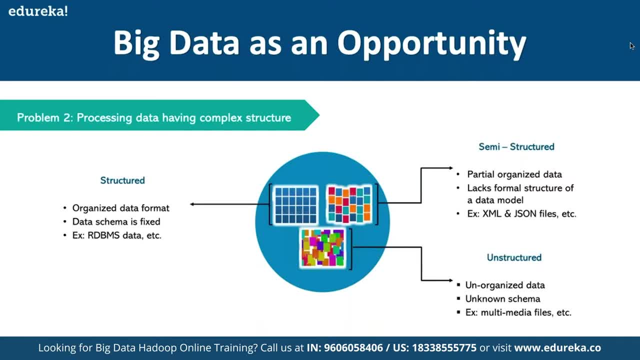 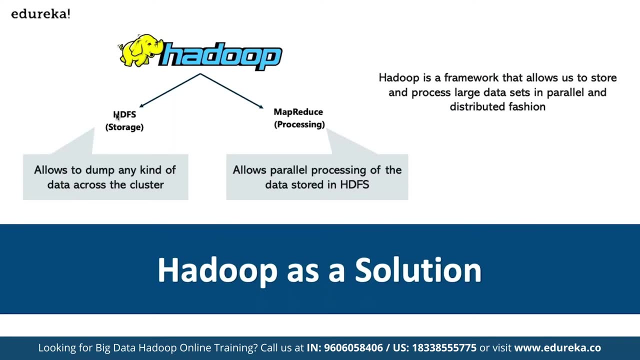 so how hadoop is offered as a solution here. so basically, hadoop allows us to dump any kind of data across the cluster and we hadoop basically has two main core components. we have our hdfs, which refers to hadoop distributed file system, and then we have map reduce, which refers to processing. 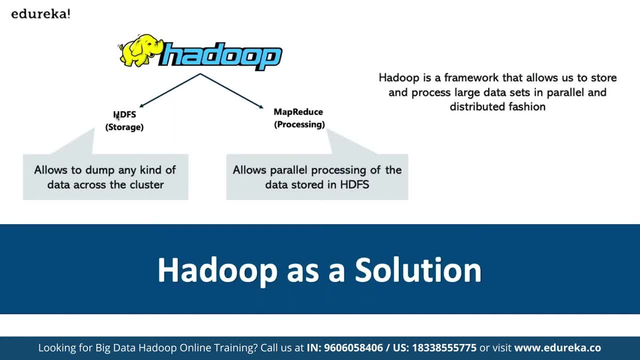 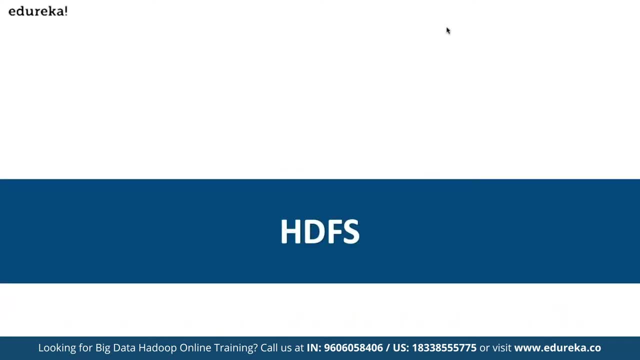 so it allows us to parallelly process the data stored in sdfs. all right. and then we have map reduce. so map reduce is basically used in combination with technologies. like we have spots, so spark is basically used for giving us the access to a real-time processing of processing, real-time stream. 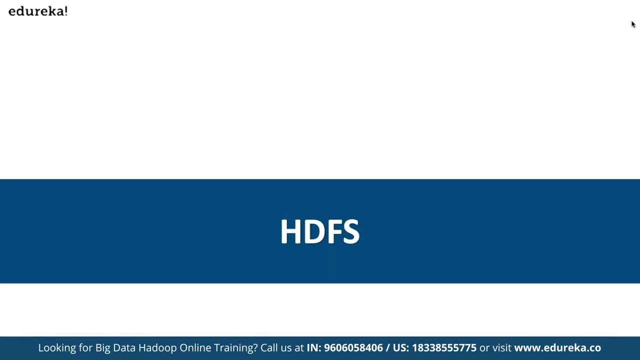 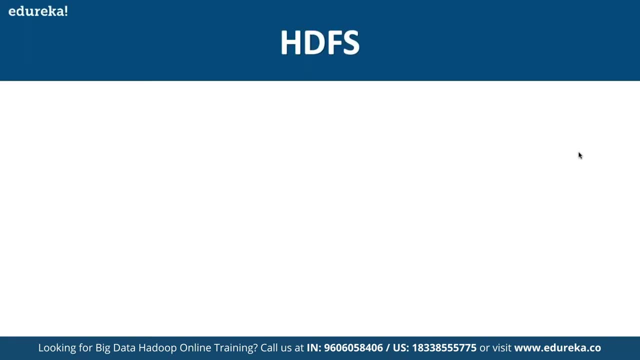 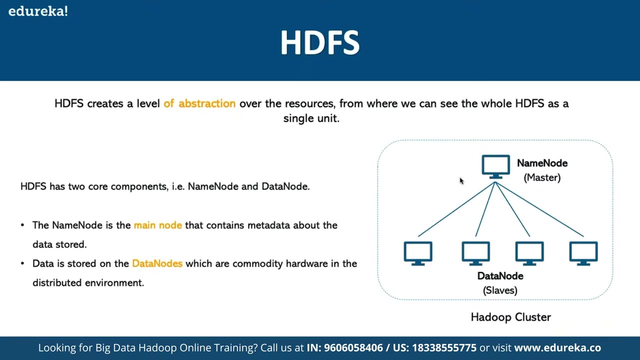 monitoring, for example, we have to do streams right. so that is what we can analyze by using these file streams. let's discuss on that. so here we have sdfs. so first of all, if we talk about sdfs- and sdfs is what it's- simply a distributed file system. so basically, here we can create a level of 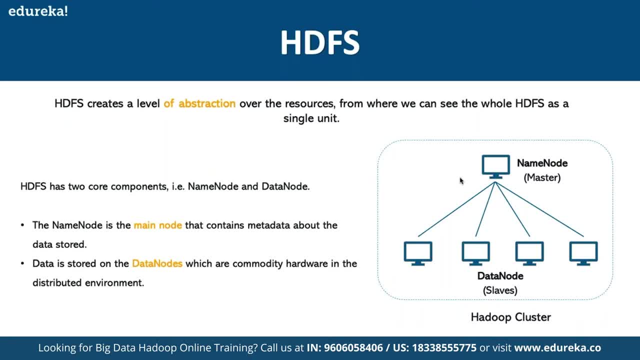 abstraction over the resources, from where we can see the whole sdfs as a single unit, and sdfs has two core components: the name node and data. so name node is the main node that contains metadata about the data stored, and then we have the data node, which are simply commodity hardwares. 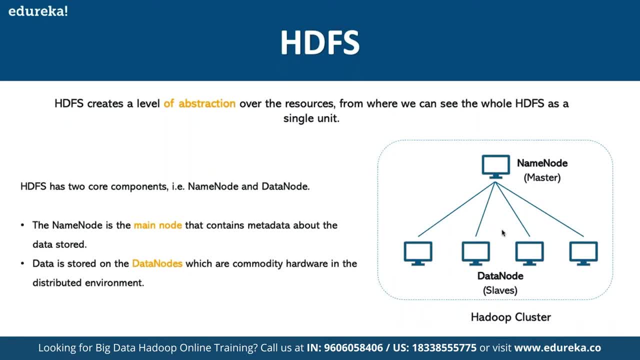 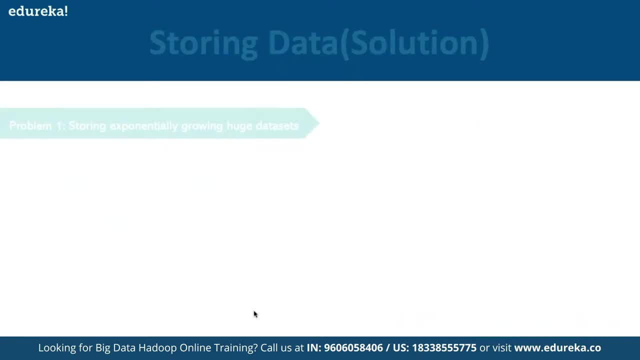 in the distributed environment. so basically, under name node we can simply create multiple data nodes, because rdm processing is something that has to be done in a cluster. we don't, we are not going to do the entire processing in a single go correct by a single system. multiple systems, they all have to. 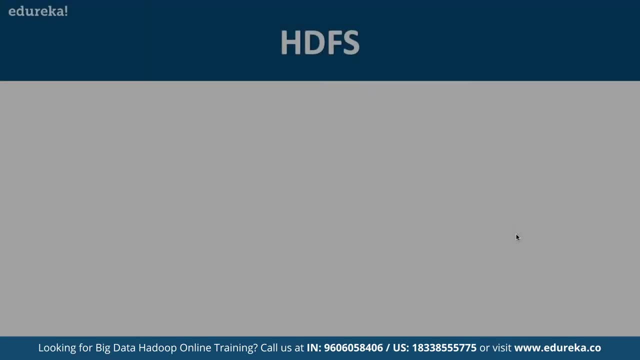 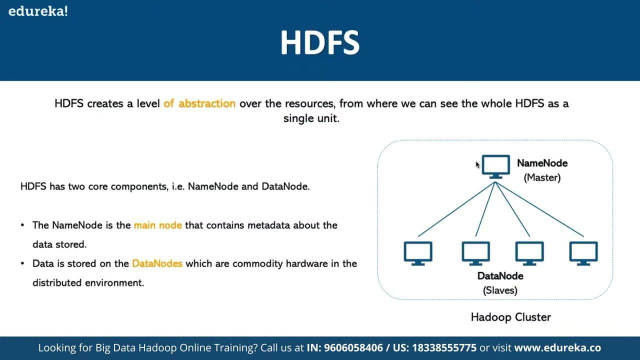 work parallelly to work on data processing, and that is what is done by sdfs. here we have a master node which simply define: okay, how many clusters are going to be defined, how many clusters are going to be created, and that's how it is going to work. so name node is a main node and the actual data 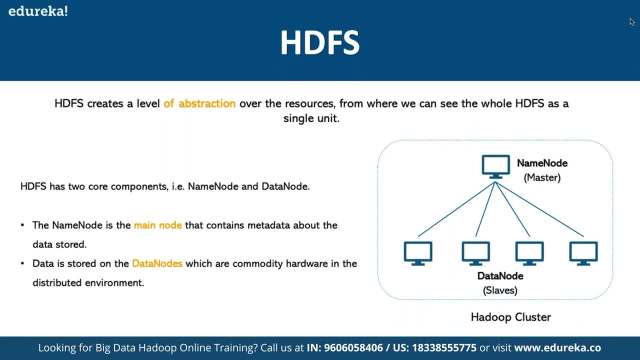 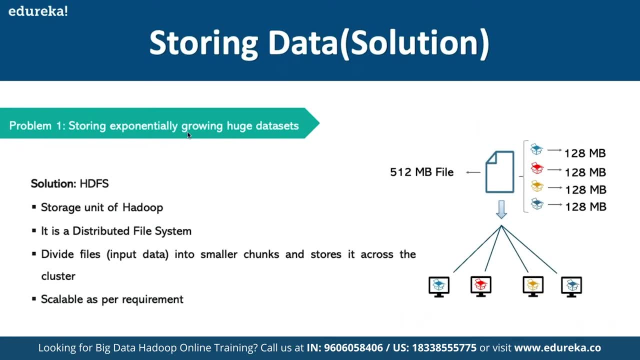 is being stored across different data nodes here. that's how it works, all right. so next we have storing data as a solution here. so when we talk about the main problem as storing exponentially growing, huge data set, the solution for that is sgfs, which is basically a storage unit of hadoop. 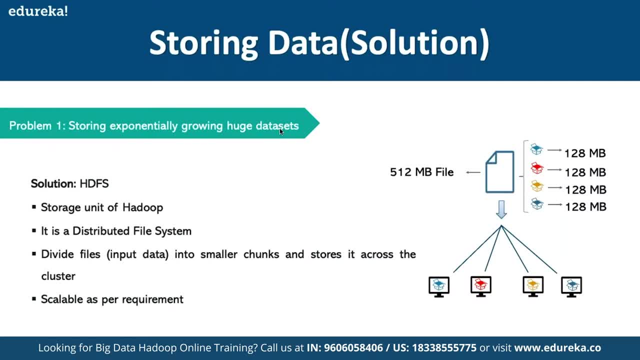 it is a distributed file system where we can divide files into multiple input data, where we have a smaller chunk, and which sorts it across the different clusters, and then we have scalable requirement. so basically, here we are going to take the requirement in terms of the mb files for 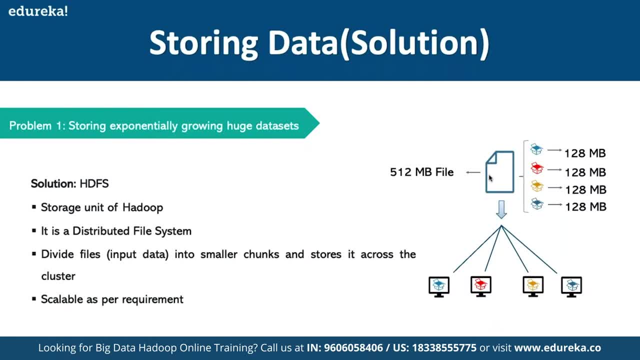 example, here we have a lot of large file as 500 mb files. so then we are going to divide this into smaller packages and then we are going to store it in different nodes so that we can process it as quickly as possible, and then we have the second problem of storing the unstructured data. so how that is solved by: 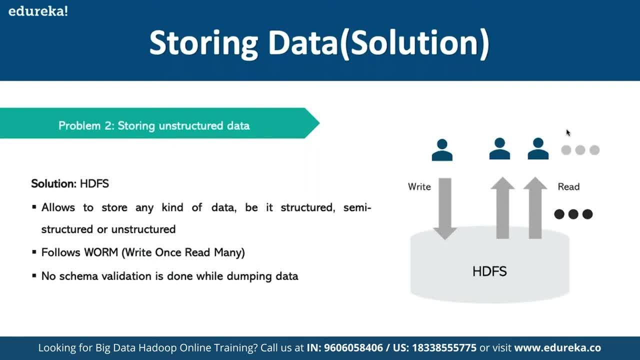 using sdfs. so sdfs allows us to store any kind of data so it can be structured, semi-structured or unstructured. so basically it forms the worm theory as in write once read many. so no schema validation is done, while dumping the data set so the users they can write data. 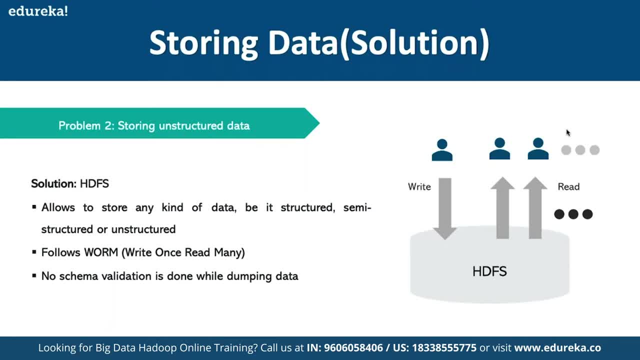 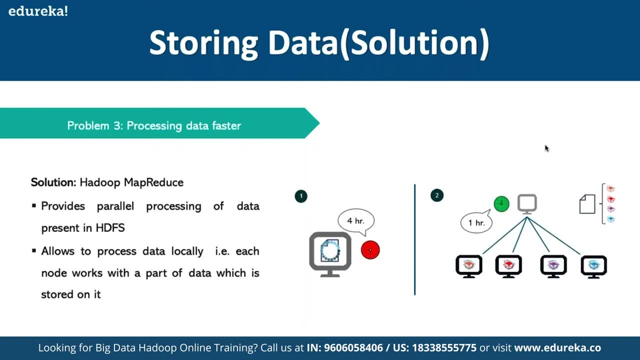 and again, multiple read operations can perform on the data that has been written on sdfs. and third problem was processing data faster. so the solution was hadoop map reduce. so it provides parallel processing of data present in sgfs, which allows us to process data locally. that is, each node works with part of data which is stored on it. so let's say, if we give a data, 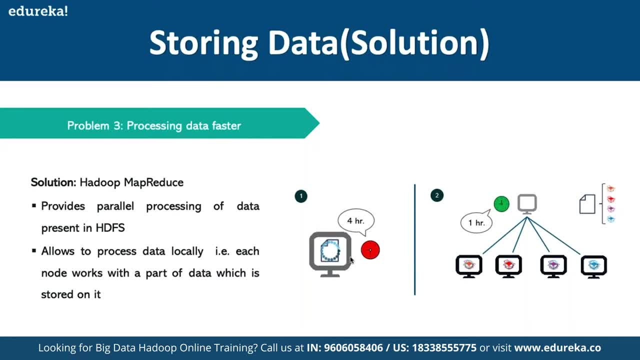 job to process 1 000 pages to a single system and we give the same job to another system where we have four connected systems and they all have a capacity of going through, let's say, 250 pages on a per hour basis. so same job is going to take four hours for the system and the same job is going. 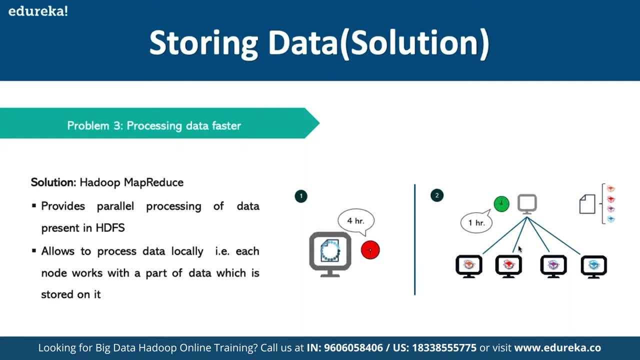 to take this one hour on the distributed system, because it seemed like the same problem statement that we have in mathematics back in our school days. if one worker is able to complete a building, then how many that? how much time will three workers take to complete the same building right? 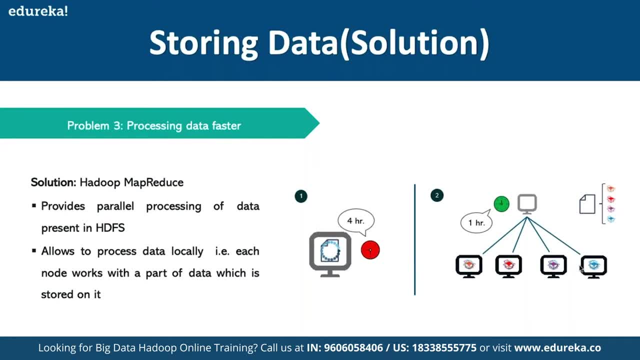 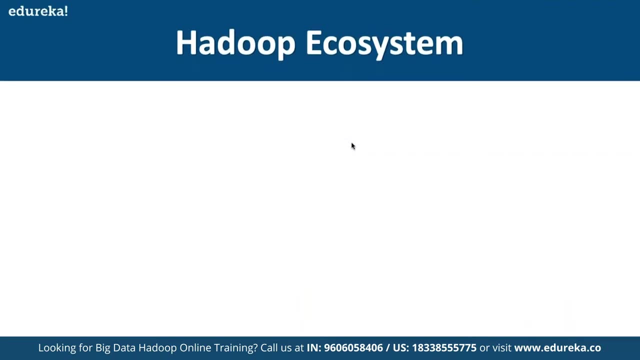 so same thing is being done here. we are dividing the work into multiple workers so that it can work faster and then we can get the output as quickly as possible. all right now. next we have the hadoop ecosystem. so, as we discussed, hadoop is basically divided into sgfs and again there. 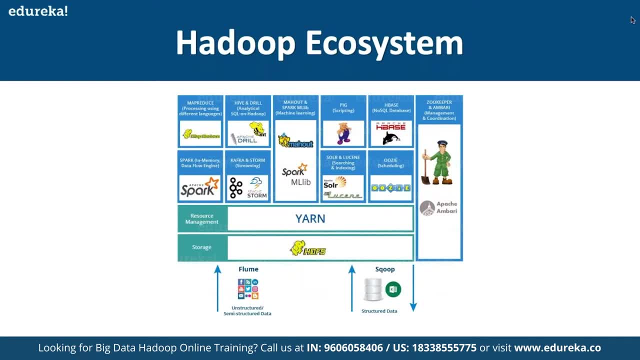 are multiple systems available under hadoop. so here we have multiple components that we have map reduce. so in map reduce again we have. so basically map reduce is used for a quick- we can say quick- batch processing and that is for handling the real-time systems same way as spark. 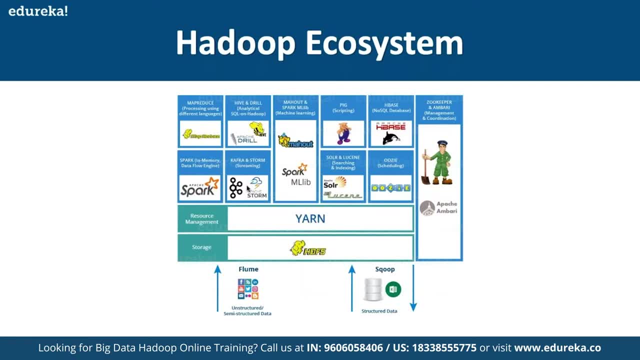 and then we have the kafka system, which is basically used as a message processing system along, which is meant to be used along with spark. so basically, for flume is something that we use for the unstructured and semi-instructed data set. you can see that we have a lot of systems available under hadoop, so here we have multiple. 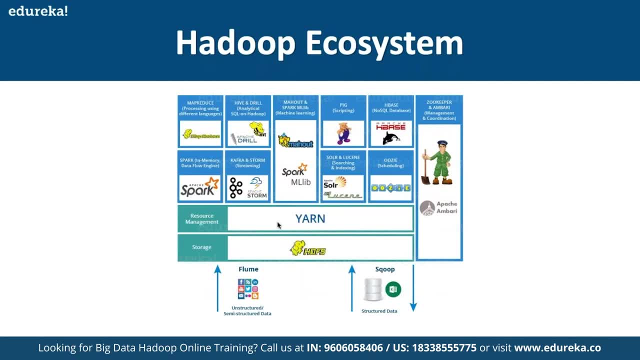 and then we store the data. on the sgfs component for resource management, we use a yarn resource manager and then we have spark, we have kafka, we have my house, which is as a part of machine learning libraries, we have big for scripting, then we have edge base, which is basically used.